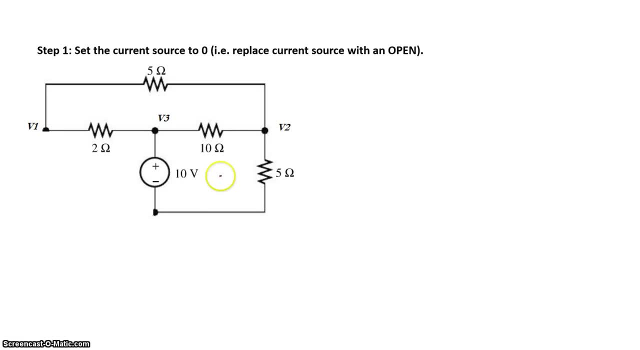 have a current source here. we open that and that wire is gone. So here's the circuit now. Now on this circuit we have the 10 volt source, a 2 ohm resistor. Now, if you look carefully, this 2 ohm resistor is in series with this 5 ohm resistor. So let's. 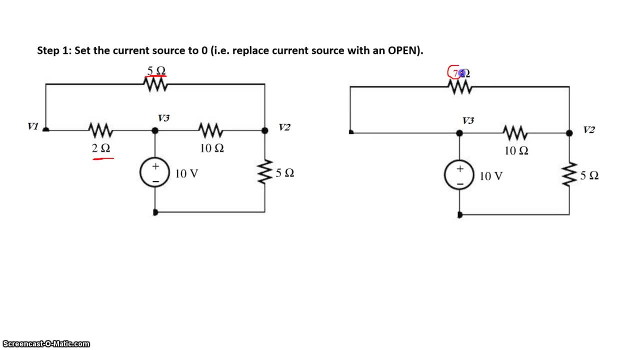 replace that with a single 7 ohm resistor right here. So that's our combined 7 ohm resistor. If we look carefully again, this 7 ohm resistor is between nodes V3 and V2.. So if you look at V3, that's on one side of. 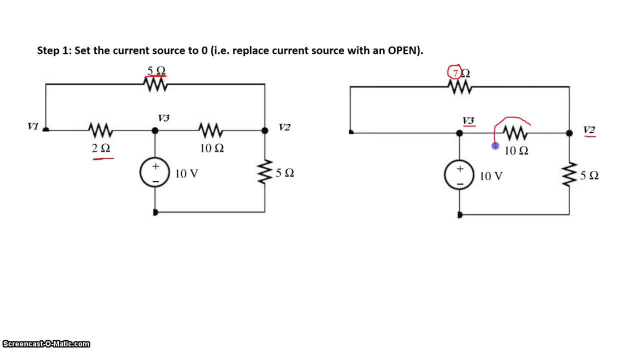 7 ohm V2 is on the other side. Similarly, this 10 ohm resistor right here is in between nodes V3 and V2.. By resistors, when they're on, when a resistor has the same two nodes on two sides, those resistors are. 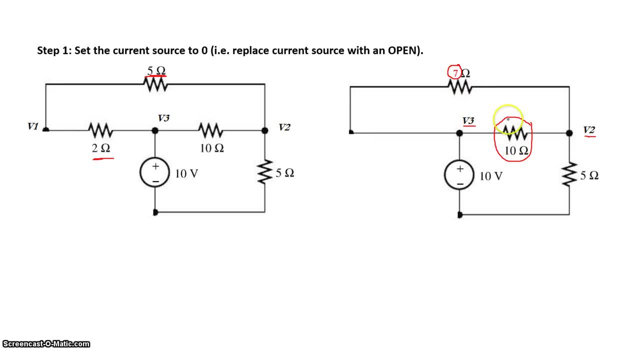 in parallel. In other words the 7 ohm and the 10 ohm resistors are in parallel. So we get, using the resistor parallel formula, we get 7 times 10 divided by 7 plus 10. So we get a combined resistor of 70 over 17.. Now we can find the 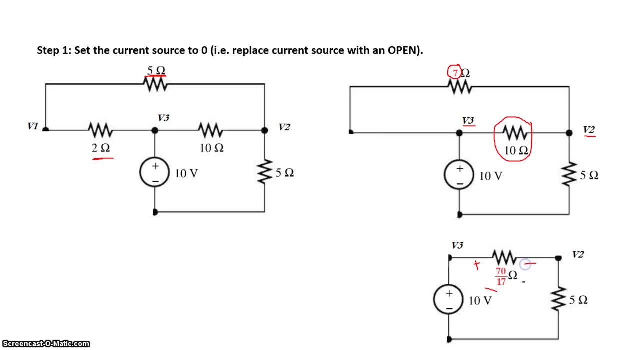 voltage. drop across this 70 by 17 ohm resistor using voltage divider. And let's use voltage divider and we get voltage 3 to V3 to equals this resistor 70 over 17, divided by 70 over 17, plus the 5 ohm resistor. 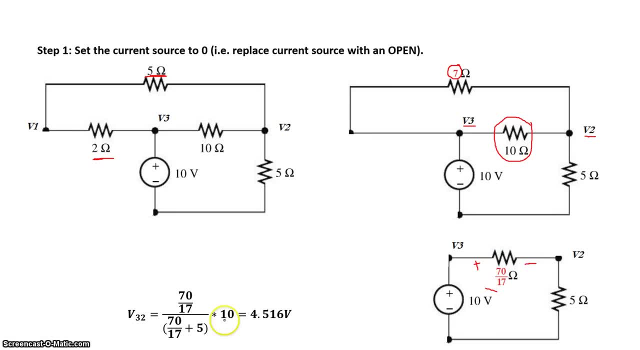 which is in series, And the total voltage that's being divided is the 10 volts. So we get 4.516 volts between nodes 3 and node 2.. So let's go back to our circuit where we started from. We have V3, V2.. The voltage drop between this node. 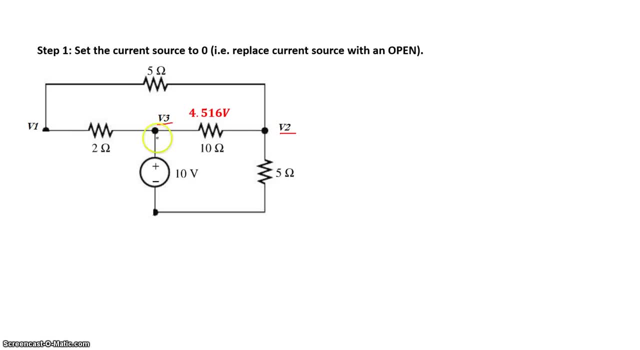 that's between 4.516.. If we look carefully, the 2 ohm resistor and the 5 ohm resistor are also between V3 and V2.. So, in other words, the 2 ohm resistor and the 5 ohm resistor are going to divide the 4.516. 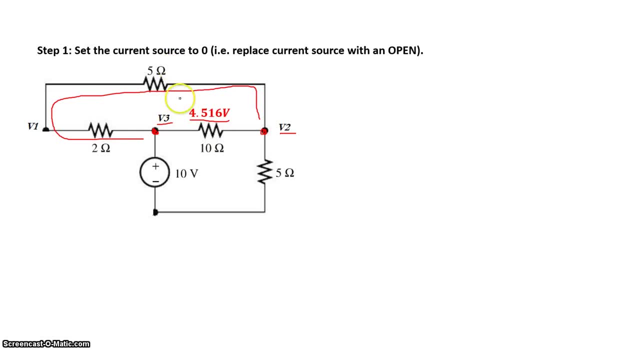 resist volt proportionally between these two guys. So let's do voltage divider there. In order to figure out the voltage drop between these two nodes or across 5 ohm, we need to basically write down: V12 equals 5 ohm divided by 5 plus the 2 ohm. that's in series times, the 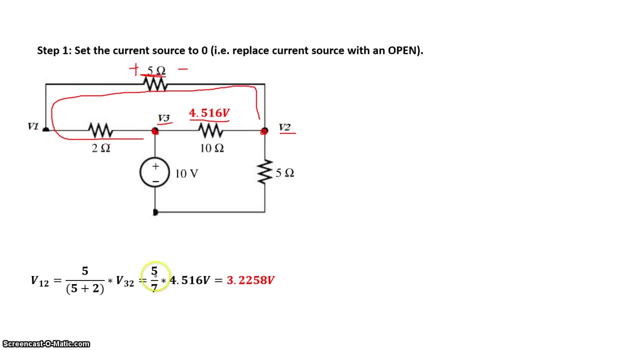 total V32.. In other words, 5, 7th of 4.516 volt, which is 3.2258 volt. Now this voltage right here is the total contribution of the 10 volt source on the voltage across this 5 ohm resistor. So we figured out what happens to the 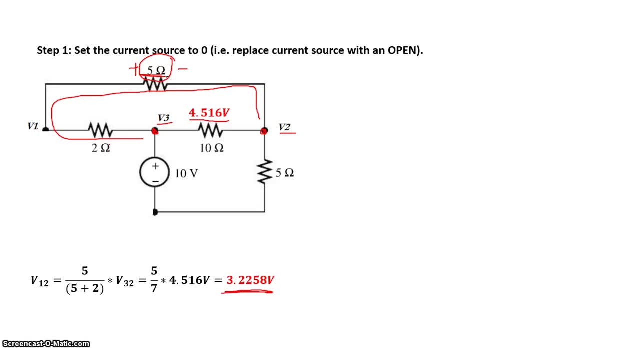 voltage across this 5 ohm resistor if the current source is not present. Now let's do the same thing, but this time let's remove the voltage source and find the contribution of the current source. So here it is Replacing a voltage source. 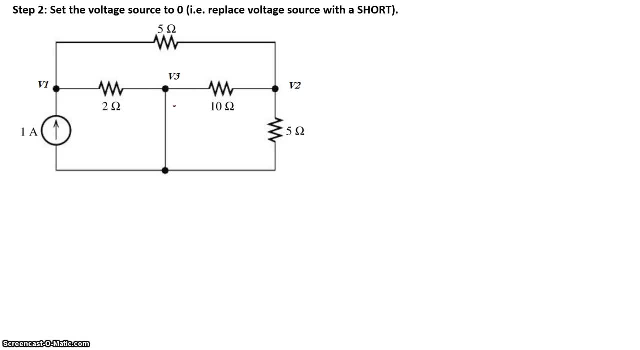 basically means setting the voltage source to zero. In other words, we replace a voltage source with a short. When we have this now? let's take a look at this very carefully- We basically have a 10 ohm resistor between node V3 and V2.. A 5 ohm resistor is also between the nodes V2 and V3. Look. 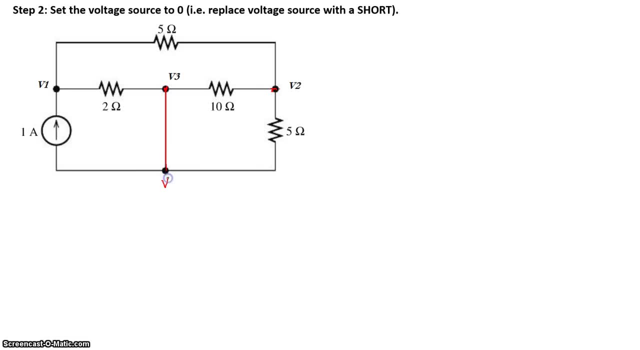 at this, because this is a straight wire. This node is also V3.. This is a 5 ohm resistor between V2 and V3.. In other words, the 10 ohm and the 5 ohm resistor are in parallel with each other. So 10 times 550, divided by 10 plus 515.. So this 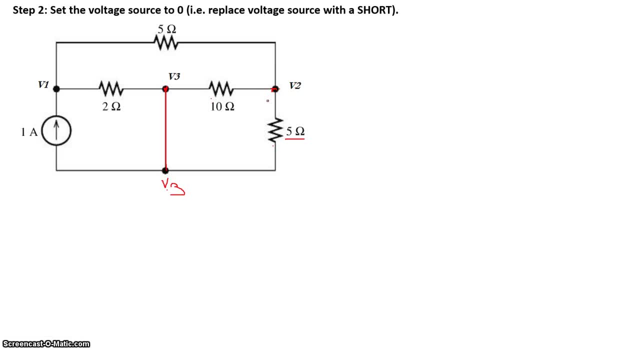 can be replaced with a single resistor between node 3 and 2.. As follows: so 50 over 15.. Now you look carefully, We have 1 ohm coming into this node. We'll call this current I2 and that current I1.. I1 travels through the. 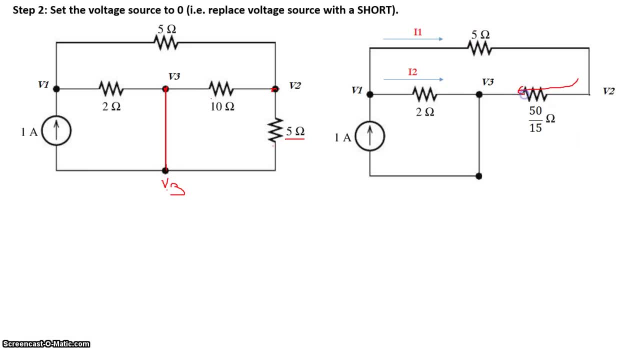 5 ohm resistor and the 50 over 15.. In other words, 5 ohm and 50 over 15 are in series. I want to use current divider as the current comes into this node In order to do that. the current I1,, since it travels. 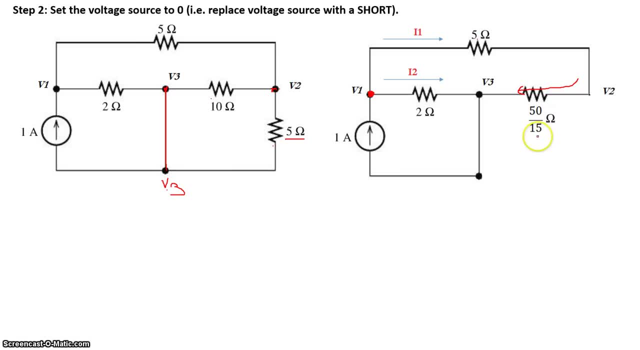 to both 5 ohm and 50 over 15, let's combine them together into a single resistor. So 5 plus 50 over 15 gives me a total of 8.33 ohms. So here we have 8.33 ohms. Now current 1 amp is coming in. It's going to divide. 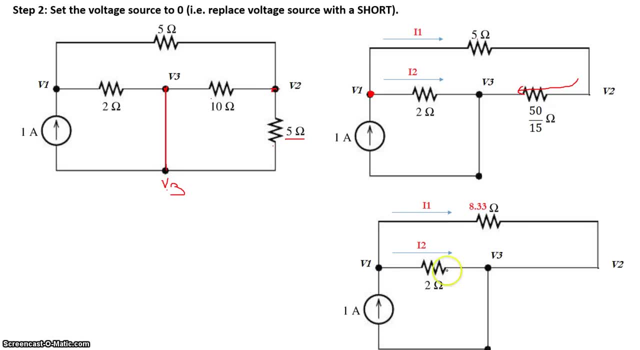 proportionally between I2 and I1 based on the size of this resistor, And if we use the current divider formula we get: the current I1 is equal to 1 over this resistance. right here: 8.33 divided by 1 over 8.33 plus 1. 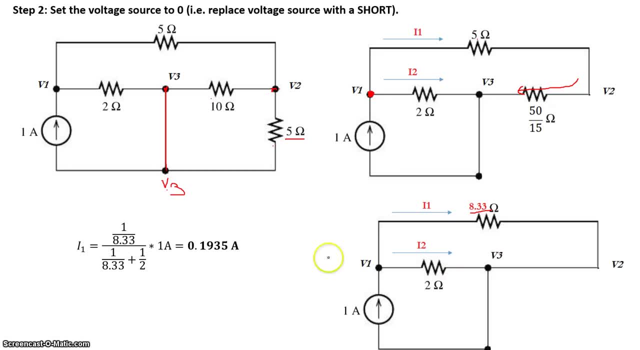 half The 1 over 2, this resistor right here. So I1 is 1 over 8.33 divided by 1 over 8.33, plus 1 half times what is being divided is 1 amp. So we get a total of 0.1935. 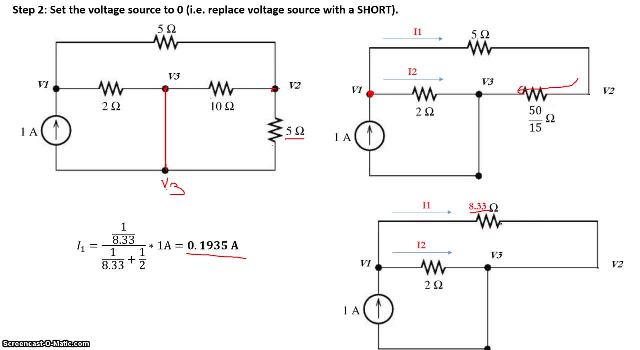 amps going through the 8.33 ohm resistor. If you remember carefully right here let me redraw that picture again- that I1 is equal to 0.1935. it's going to the 5 ohm resistor, so the voltage across. 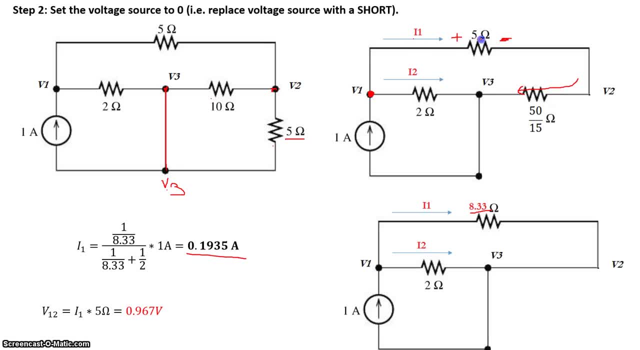 this 5 ohm resistor can be calculated by I1 times 5 ohm, so I1 times 5 ohm, which leads me to 0.967 volts. so if we figure out the voltage across this 5 ohm resistor or this 5 ohm resistor, when the voltage source that was present here was 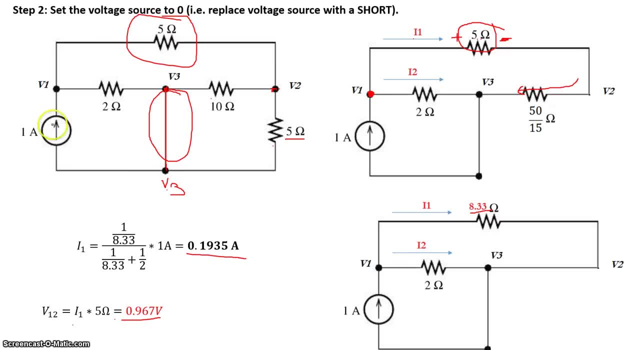 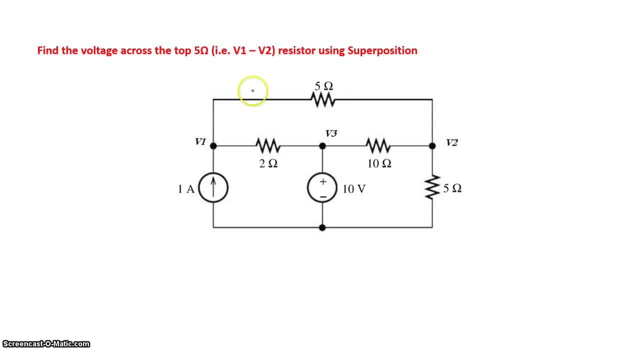 removed. so we figured out the voltage drop across a 5 ohm resistor because of this 1F current. so now so in this original circuit we figure out that the voltage contribution from the voltage source is 3.2258 volts. the voltage contribution from the current source is 0.967 volts, so by 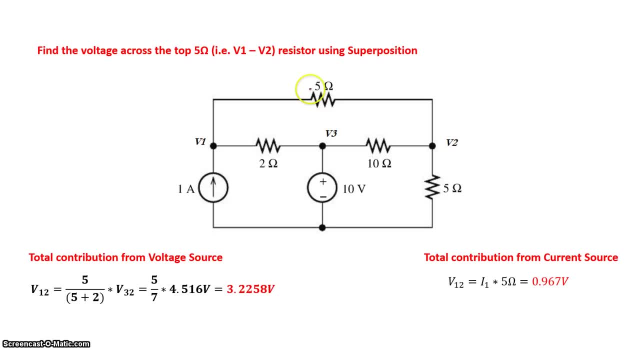 superposition, the total voltage across this 5 ohm resistor is equal to 3.2258 to 58 plus 0.967. so that leads me to, by superposition, it leads me to four point one, nine, three, five volts, or in other words four point two volts. okay, that is. 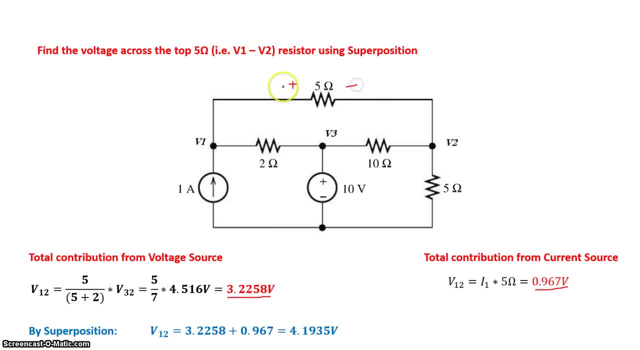 the total voltage drop between plus V 1 and V 2 and that is four point two volts total. so that's the concept of superposition.